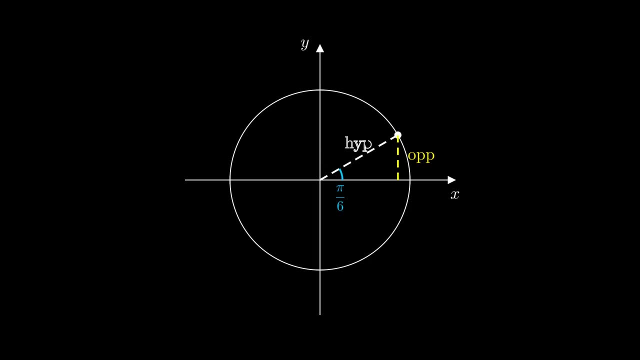 The sine function can be defined as the opposite, divided by the hypotenuse in this right angled triangle, or if we're in the unit circle which has radius 1,, it's just the length of the opposite side, which is the y value of this point on the unit circle. Now look at this regular hexagon. 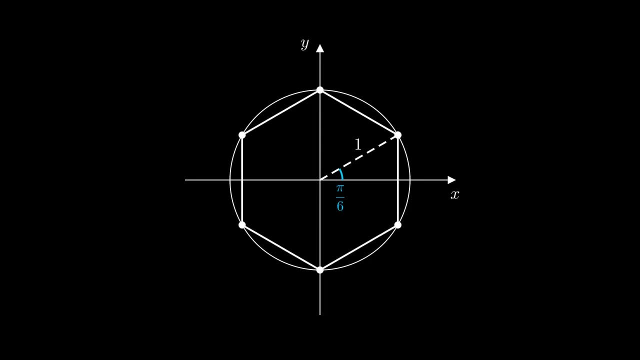 It's inscribed in the unit circle. so the distance from the centre to the vertex is 1 and the sine of pi on 6 is half the side length of the regular hexagon. We can find the length by focusing on this triangle. All the angles are pi on 3 or 60 degrees, so it's equilateral. This side length is 1. 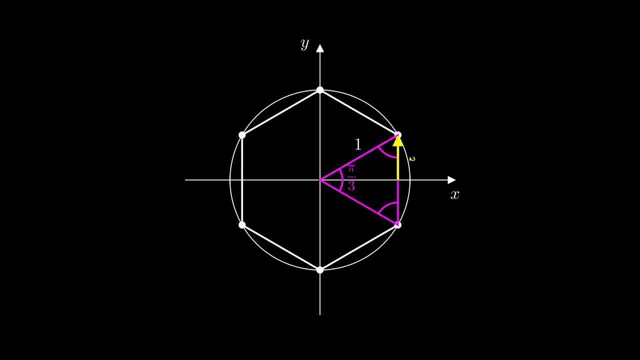 so the sine of pi on 6, which is half of one of the side lengths, must be equal to 1: half, If you're okay with that. now let's do a similar thing for the sine of pi over 5.. We can represent it on the unit circle and because it's 1 fifth the way around to pi. 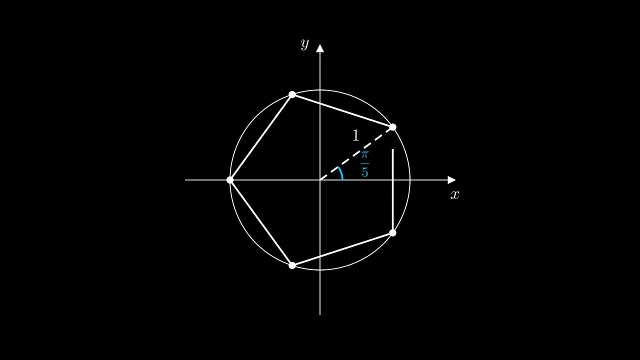 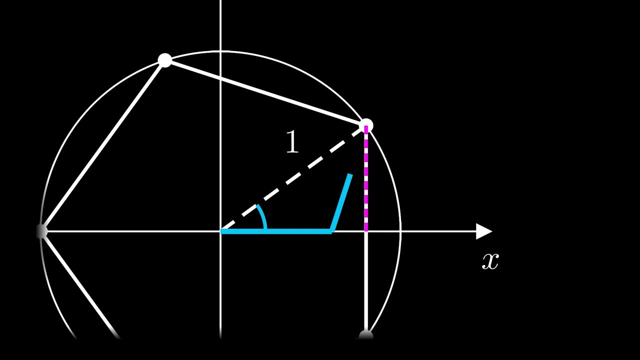 we can inscribe this regular pentagon and the sine of pi on 5 tends out to be this length. here We can calculate it by constructing some isosceles triangles, Let's say these blue line segments all have length a. What we've constructed 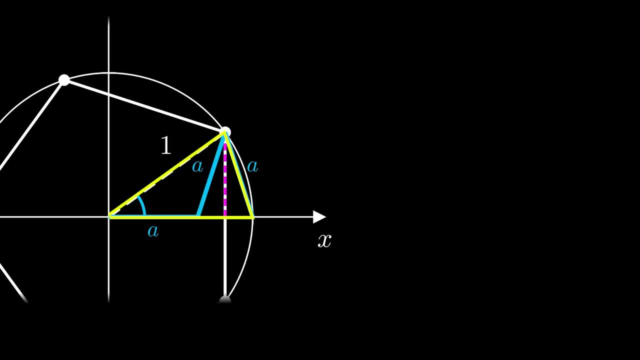 there is called a golden triangle. It's an isosceles triangle with 1 angle of pi on 5 and 2 angles of 2 pi on 5 or 36,, 72 and 72 degrees. It's more famous cousin is the golden rectangle. 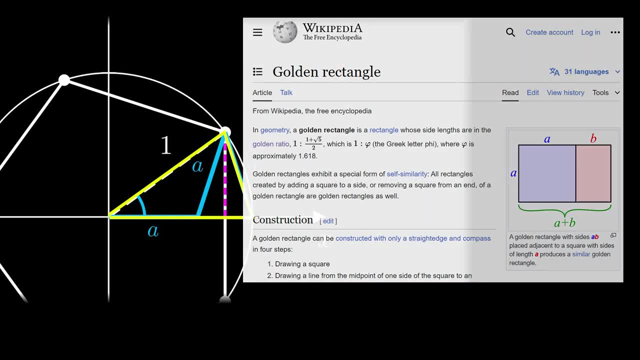 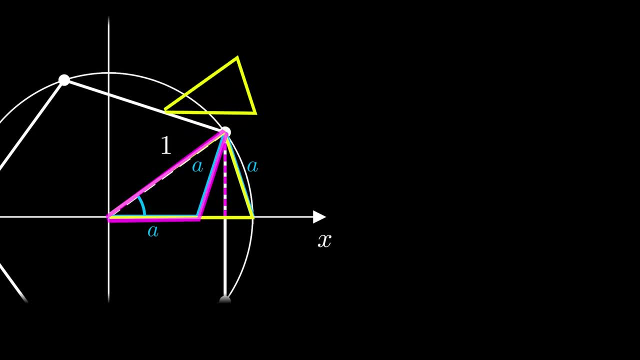 where, if you cut out a similar golden rectangle, you're left with a square In the golden triangle. you can cut out a similar golden triangle and you're left with an isosceles triangle. In similar triangles, the ratios between side lengths must be equal. We. 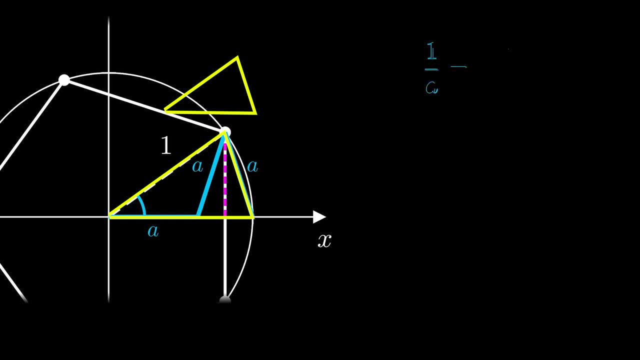 can use that fact to set up this ratio. 1 divided by a must be equal to a divided by 1 minus a. Then solve for a using the quadratic formula, Which would give two solutions, but we know it must be positive, so we just take this. one Turns out to be 1 over the golden ratio phi. 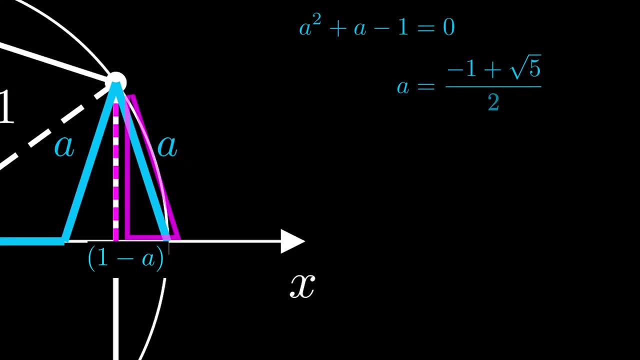 Finally, we can use this right angled triangle Applying the Pythagorean theorem gives the square root of a squared minus 1, minus a over 2, all squared. There is a bit of arithmetic expanding the brackets and collecting the like terms, But we can simplify it down to this, which. 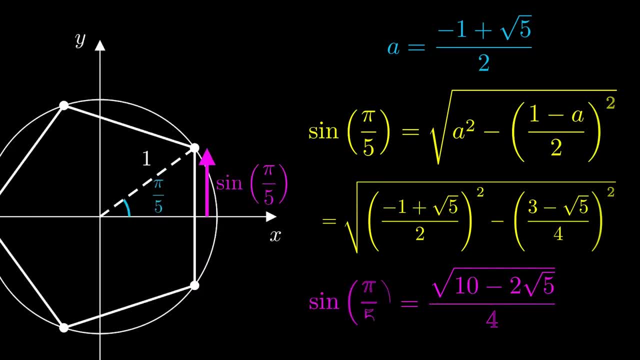 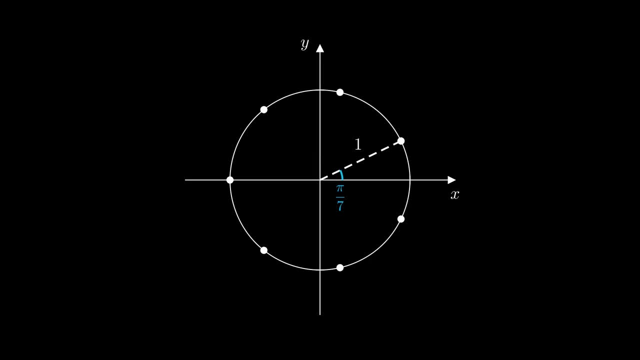 gives the exact value for sine of pi on 5.. Nice, I think it deserves a thumbs up. But you might be wondering about pi over 7.. Couldn't we do a similar thing to find this exact value? And actually the answer is no, Of course. sine of pi over 7 is a real number. 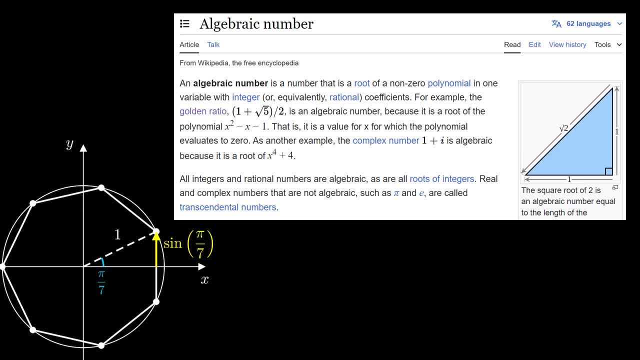 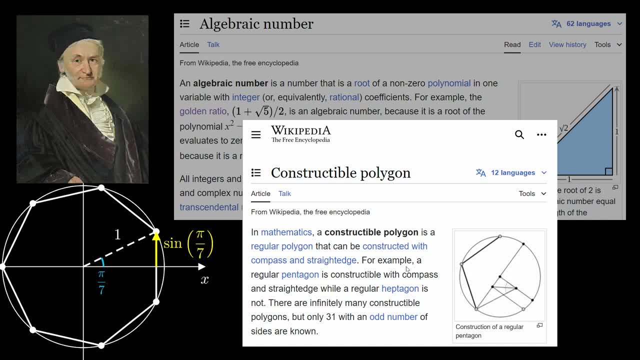 it's this length here, But the 7 sided regular polygon is not constructable, meaning it cannot be constructed with a straight edge and compass. This relationship was studied by Gauss, the prince of mathematicians, when he was just a teenager. One of the first breakthroughs that 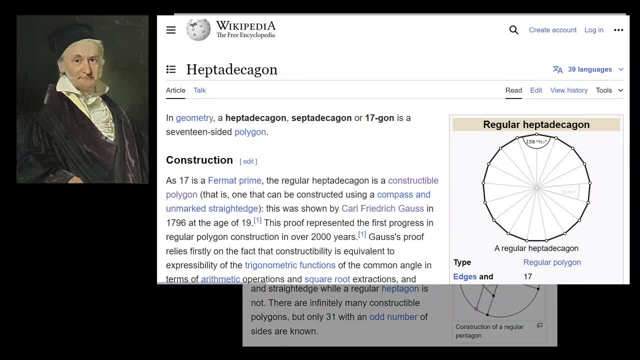 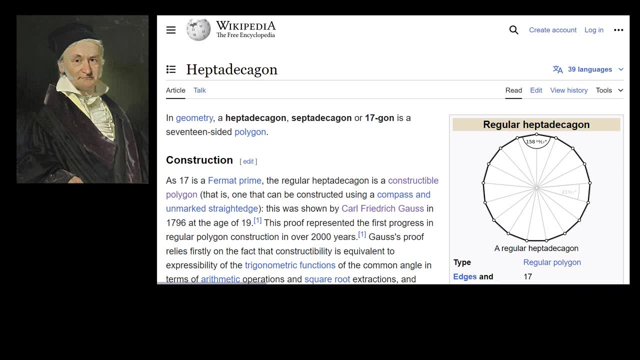 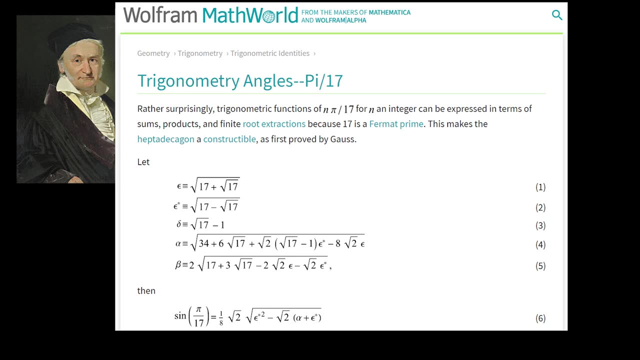 made him famous was proving that the 17 sided regular polygon is constructable, Which means that sine of pi over 17 is an algebraic number. it can be expressed in terms of roots, A lot of roots. Gauss proved that the 17 sided regular polygon is constructable because 17 is a firm. 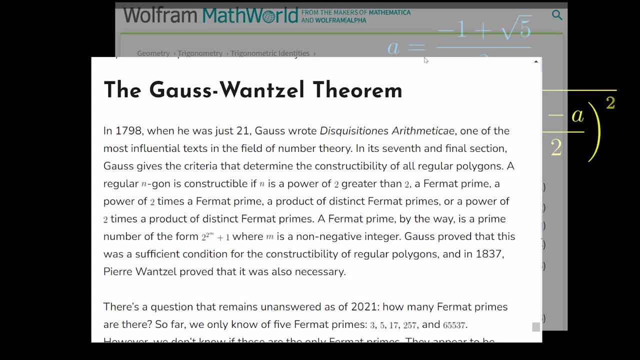 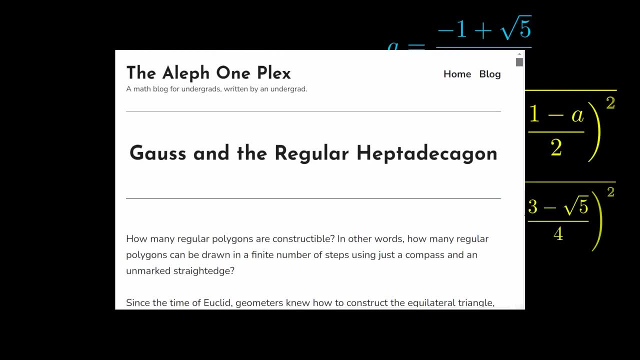 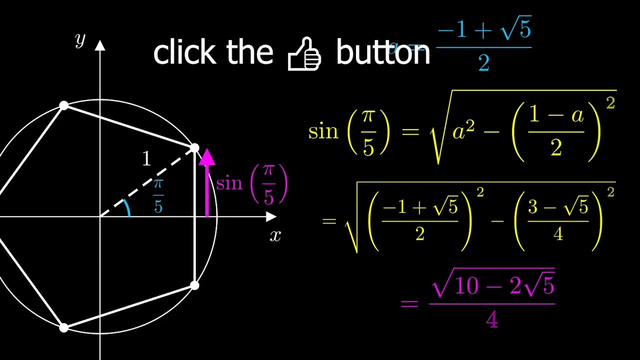 R prime. His work was built on later by Pierre Wenzel, and now the result goes by the name of the Gauss-Wenzel theorem. There's a really nice article about it, which I'll link to below. leave a thumbs up on the video before you go.